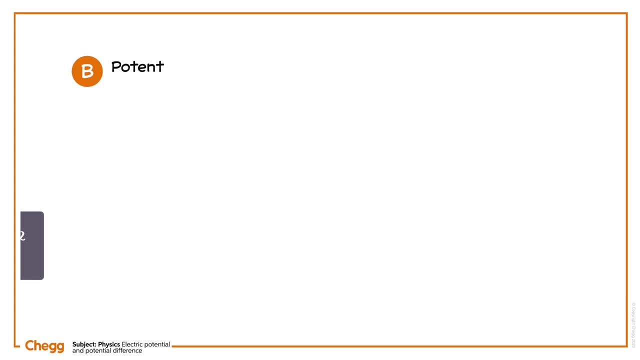 The second term we'll introduce in this video is potential difference. Potential difference is simply the difference in electric potential V between two points, and it's more commonly known as voltage. Consider two points, A and B, at the same point. We'll be noodleing the device pai and per. 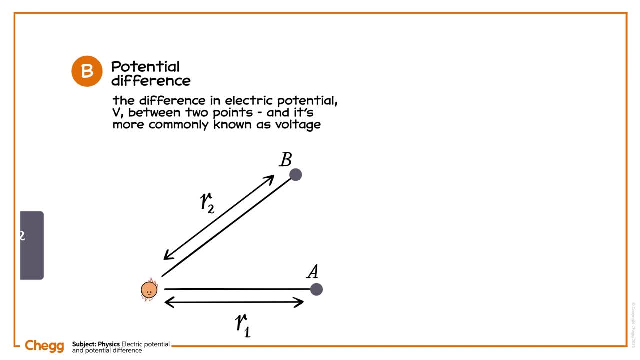 distances R1 and R2, respectively from a point with charge Q. To calculate the potential difference between A and B, we first need to calculate the electric potential at each point, then find the difference. The potential difference equals VB minus VA, which is equivalent. 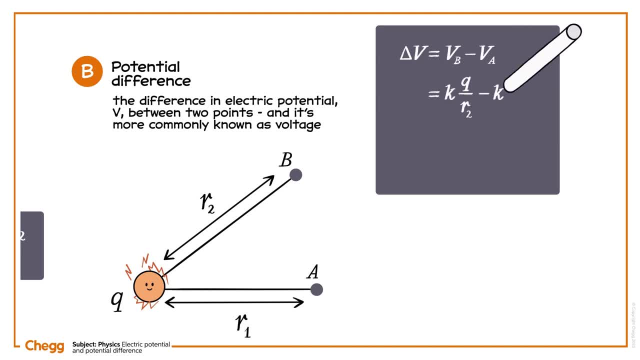 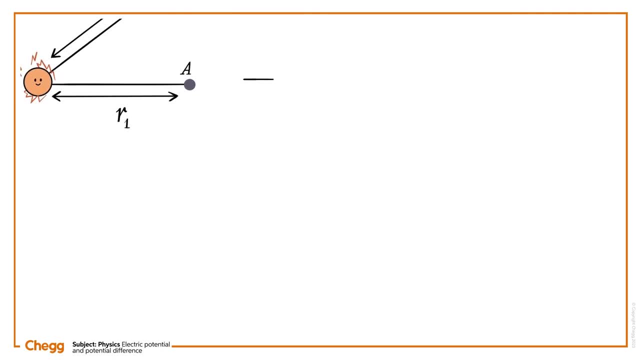 to K times Q over R2, minus K times Q over R1.. Rewriting the equation, we get this: Both electric potential and potential difference are scalar quantities measured in volts. A household battery's potential difference may typically be around 1.5 volts, while for 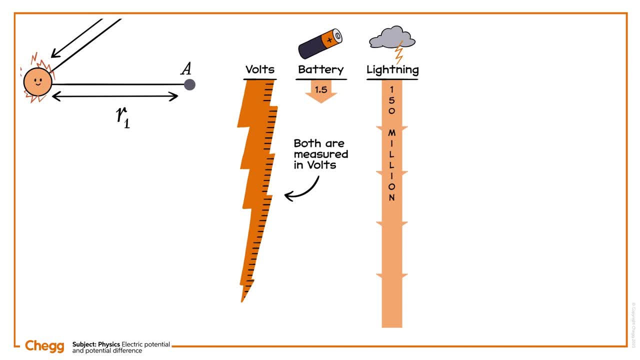 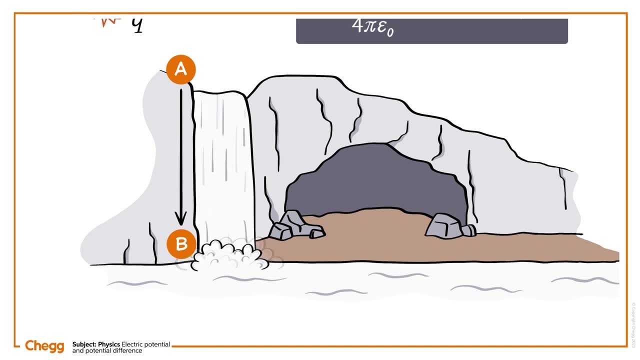 lightning. this can be as high as 150 million volts. A potential difference between two points causes movement from one point to another. It's just like a waterfall, where water flows from a higher gravitational potential to a lower one. Similarly, potential difference or voltage. 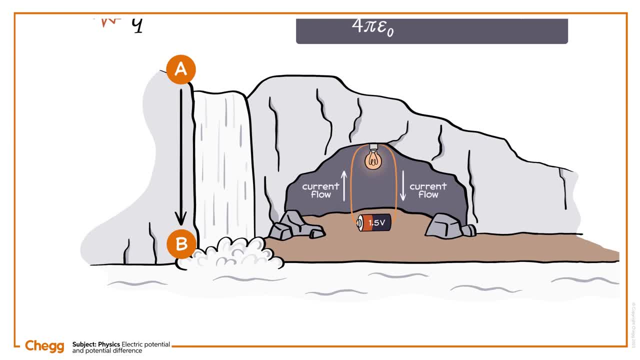 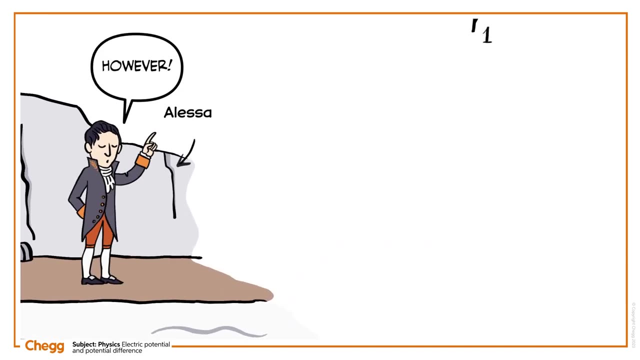 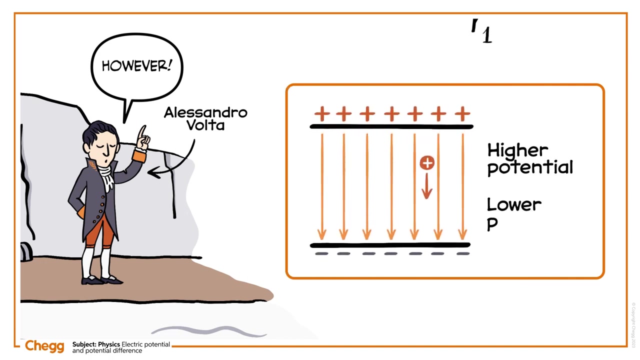 moves charges at the same time. A positive charge moves from a high potential to a low potential. but if the charge is negative, the reverse is true: The negative charge moves from a low electric potential to a positive charge. The positive charge moves from a low electric potential to a high electric potential. 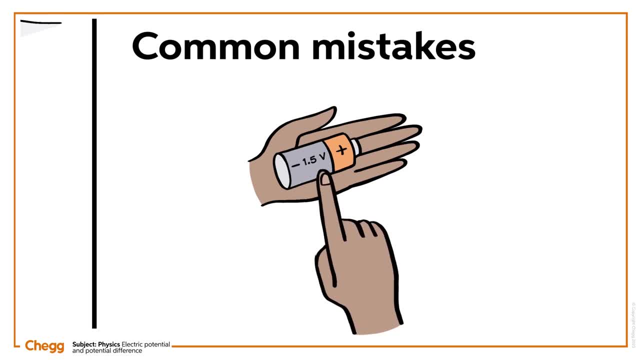 Just because one side of a battery has a minus sign and the other has a plus sign, don't assume that one has a negative electric potential and the other has a positive one. The side with the minus sign actually has an electric potential of zero volts. 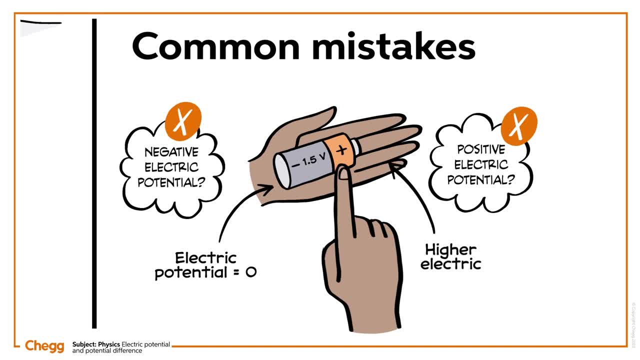 In contrast, the side with the plus sign has a higher electric potential. Therefore, the value at the plus terminal equals the potential difference between the two terminals terminals, For example, a battery being 1.5 volts, means the plus terminal is 1.5 volts.